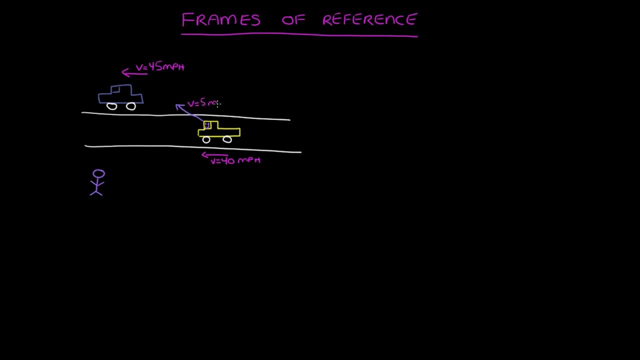 would observe the blue car traveling at 5 miles per hour. How could the person on the side of the road see the blue car traveling at 45 miles per hour and a person in the yellow truck see the blue car moving at 5 miles per hour? 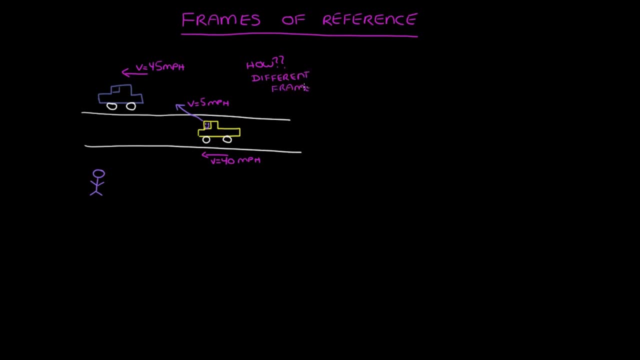 This is because both observers are using different frames of reference, So let's go ahead and take a look at that, starting with the speed of the blue car. The person on the side of the road is using their frame of reference of being at rest, So, relative to them, the blue car is moving at 45. 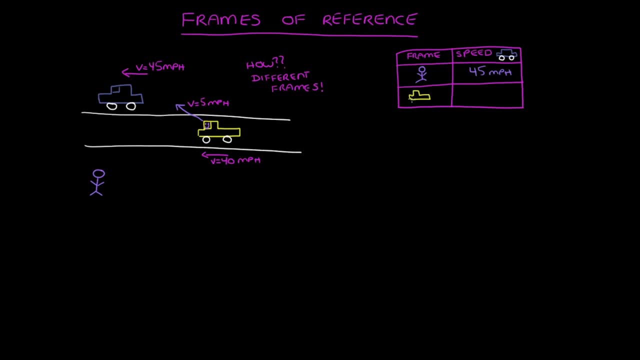 miles per hour To the person in this yellow truck which, remember, is already going 40 miles per hour. the blue car is going 5 miles per hour. Let's do the exact same thing for the speed of the yellow truck. So what is the speed of the yellow? 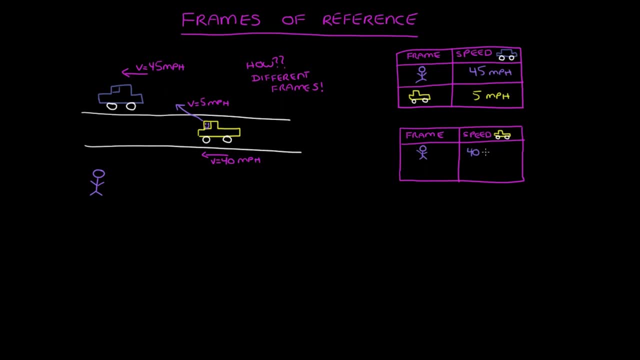 truck. for the observer on the side of the road It's 40 miles per hour, And what do you think the speed of the truck is for the person using their blue car as the reference frame? Well, the blue car is moving at 45 miles per hour and the truck is only moving at 40 miles per hour, So the speed of the yellow truck is actually 45 miles per hour. 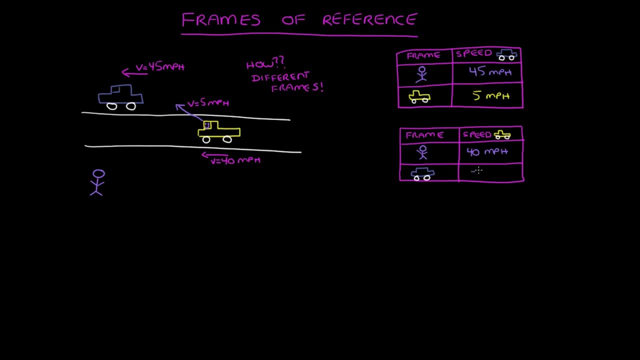 So the speed of the yellow truck is actually five miles per hour slower than this reference frame because the blue car is already moving at 45 miles per hour. Now you might be thinking: but wait, the person on the side of the road isn't really at rest, They're on the earth and the earth is. 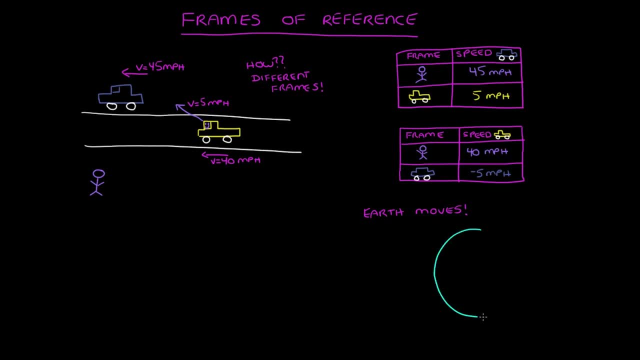 moving. You're completely correct. The person is at rest with respect to the earth, and the earth is the most common frame of reference that we use To an observer in space who is not rotating with the earth. the blue car is going 45 miles per hour plus the speed of earth's rotation. 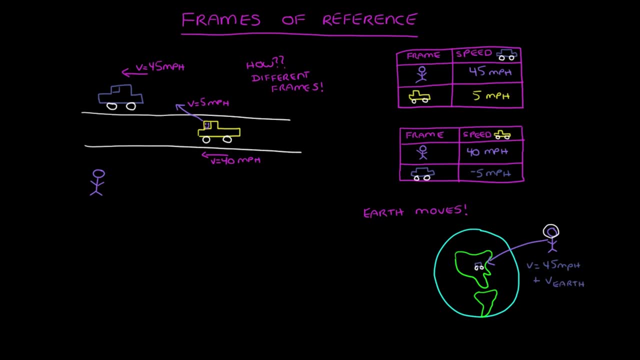 And this is why frame of reference is so important. We just talked about one blue car having three different velocities, depending what the frame of reference is. How would we communicate this to avoid confusion? Well, we state the reference frame we're using, The blue car is moving at five miles per hour, with respect to which I'll write as WRT.